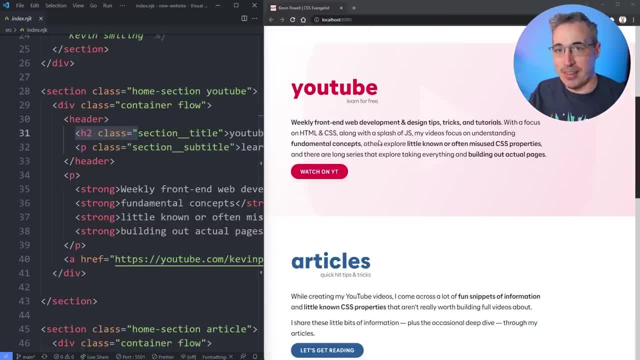 section and then I have my heading within that section and that was something I knew about and I always, I guess, assumed that it was that which gave made the section work. and when we have sections, it's like anything else with our main or with article and other things like that. 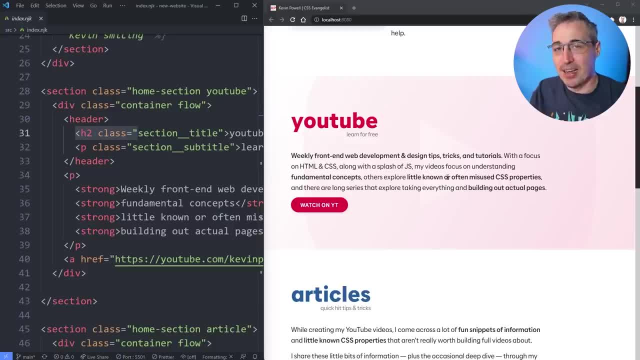 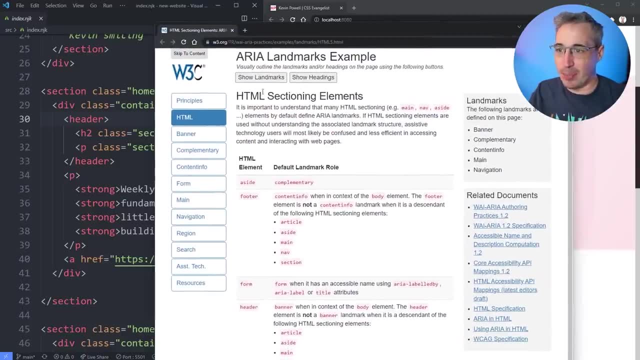 these become regions of a site or landmark regions of a site. that can really help with assistive technologies. And here we're just going to open up the W3 site- I have it just off screen and you can see here- about HTML sectioning elements and it's important to understand. you know the main. 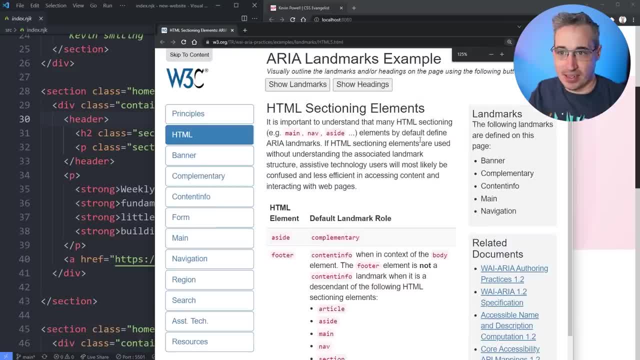 the nav the aside. it even gives the examples of there and these, as it's says they are default. by default define area landmarks and this landmark structure. I've talked about it previously, so if you're curious a little bit more on exactly what that is and why it's so important, you can watch the video. the card should be popping up or there's a link. 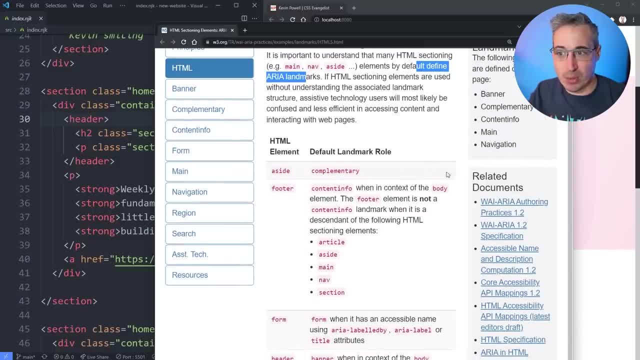 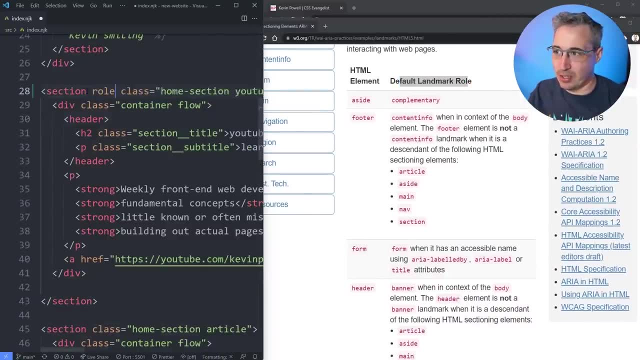 down below on exactly what that's doing. but if we come here and we look at this, the default landmark role, we have complementary. so this is- you might have seen it- where you get like a role, so I'm just going to do it- role is equal to region and the roles here are important for 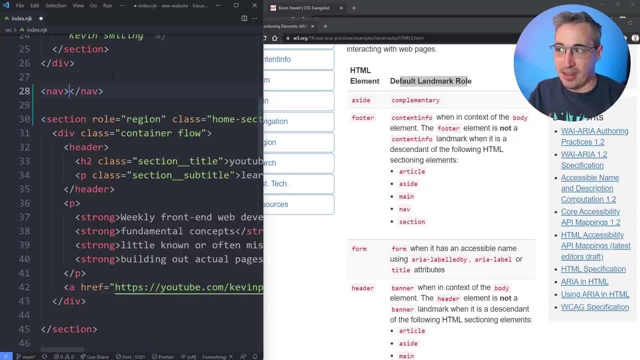 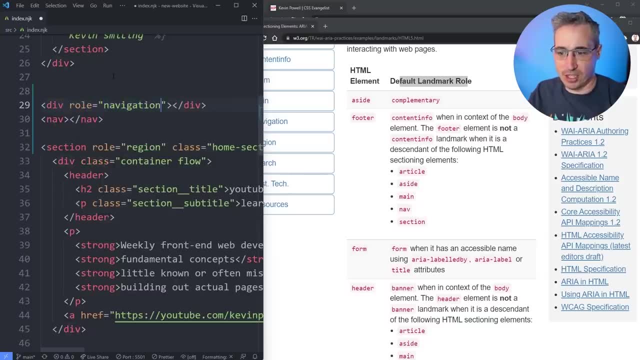 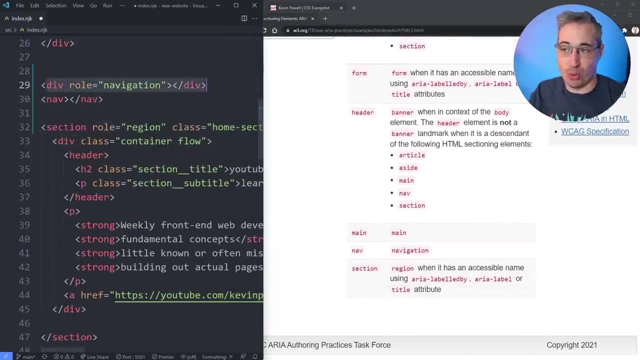 this and it's why we have like our nav right. so when you do a nav, the nav is sort of like doing a div and having a role is equal to navigation. I believe let's see. uh, there we go. so you can see, the nav is a role of navigation. so instead of having to write out, div, role equals navigation. 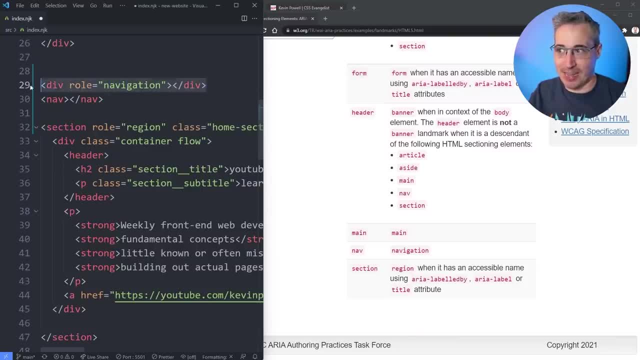 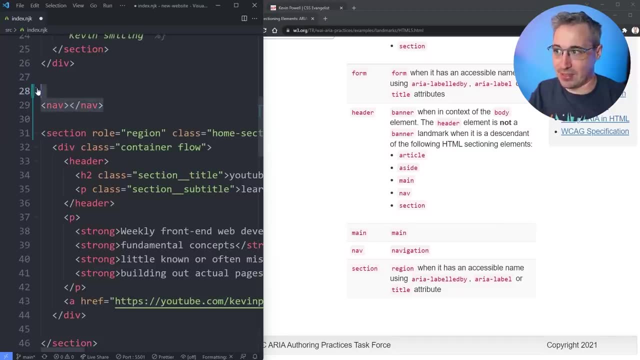 we get this role baked in just by putting nav instead. so of course we're going to do that. it makes a lot more sense and it helps the assistive Technologies know what this is. it gives it a romantic meaning sections. I always just assumed as long as you had a heading in there, they would 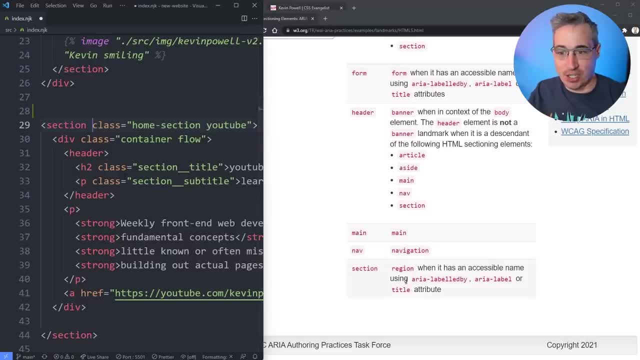 work and they would add to that. but if we see here a section is the role of region, like I just had, role equals region but that this role automatically only gets added. it's not getting added like with a nav or like with my header or like with a form and all of that it only when it has an accessible. 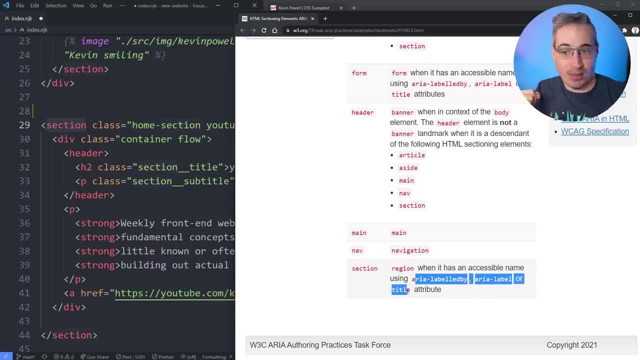 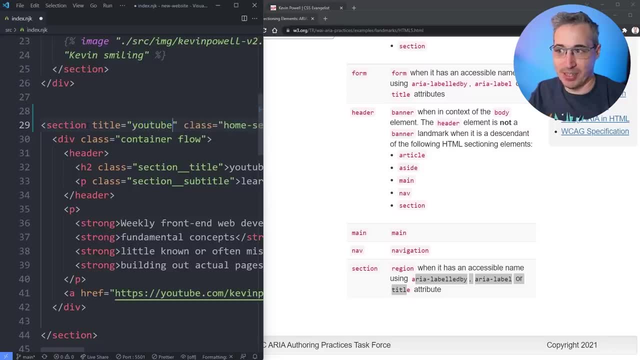 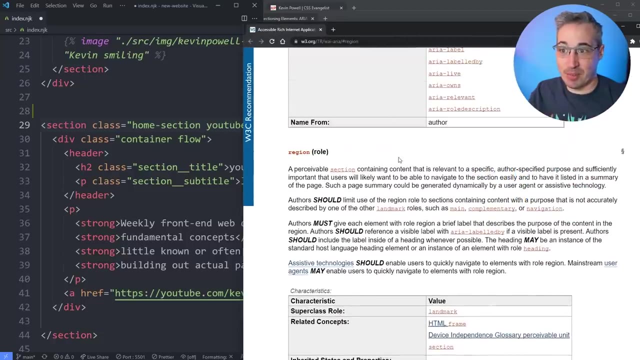 name using either area labeled by area label or the title attribute. hmm, so you can come on here and give this a title, and then this could be my like YouTube. and now this section has a title, so now it is being marked as a region, and so here is the information from the. 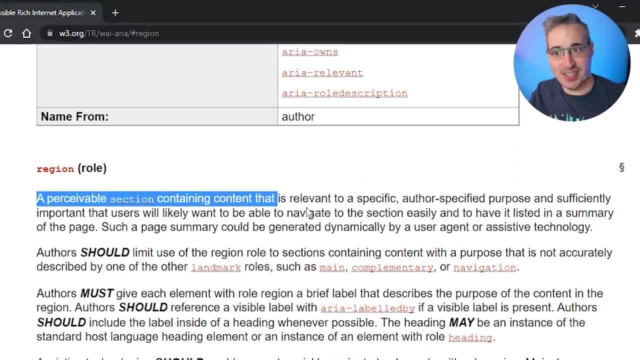 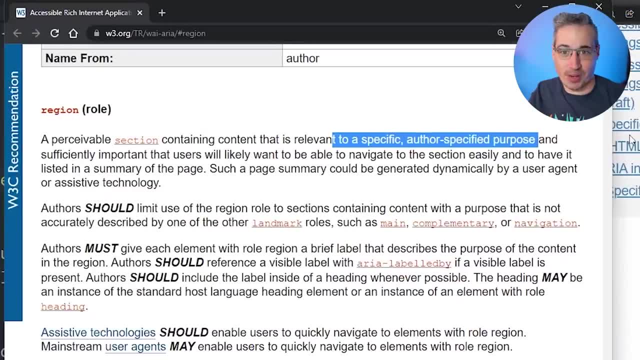 w3 on the region role itself. so a perceivable section containing content that is relevant to a specific author specified purpose, and this is sort of where the important part is. it's sufficiently important that users will likely want to be able to navigate to that section easily, and 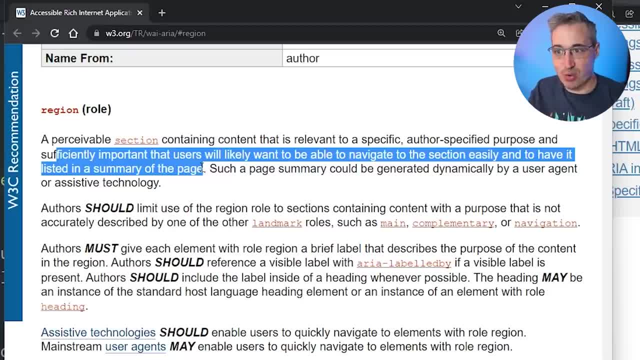 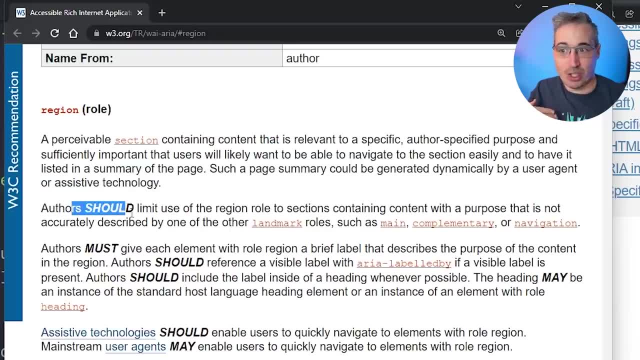 use it to create a page, because these assistive Technology screen readers. they can read the summary of a page and will include things like this: um, as it says right here. so authors should limit the use of the region role to sections containing content with a purpose that you know. 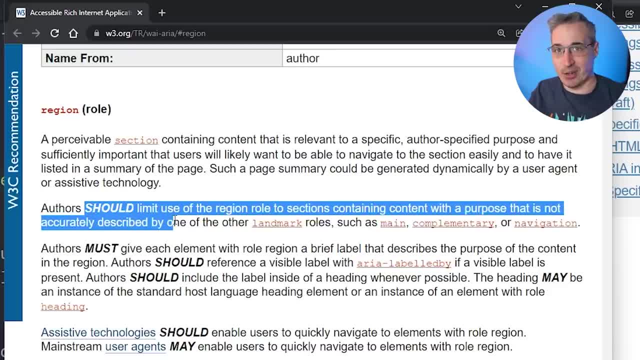 first of all, it's so. this part's just saying it should be like last case scenario. so if it's your main or your nav or your site or something like that, do those first and then, if you get to these other types of situations where there's less purpose, there's, there's not something more. 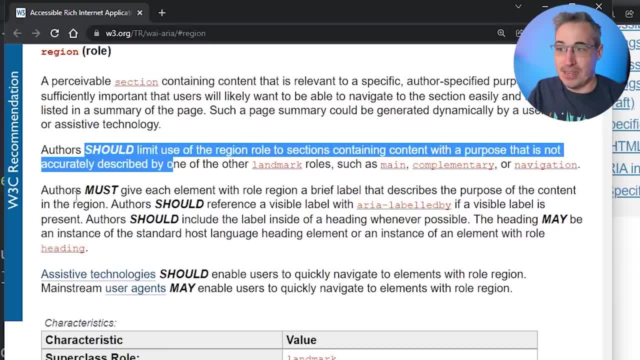 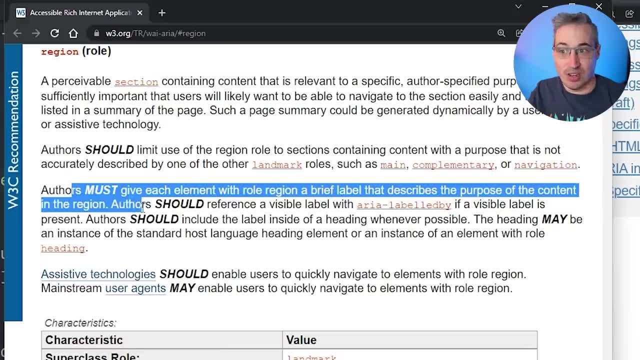 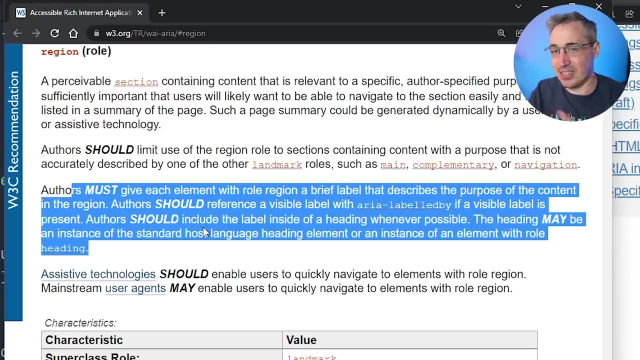 specific you should be using. then you use your section, but authors must give each element with a region rule a brief label that describes the purpose of the content of the region. authors should reference a visible label with area labeled by if one is present. so here they are saying: don't use the title. the title. 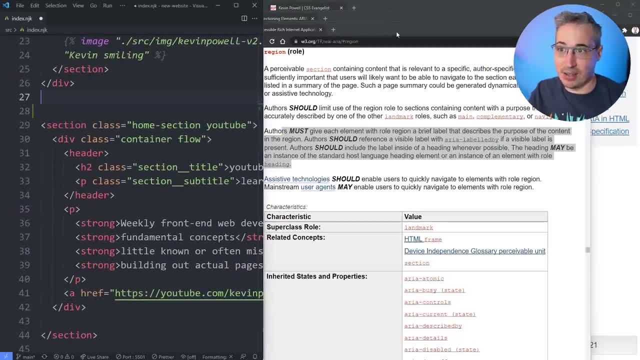 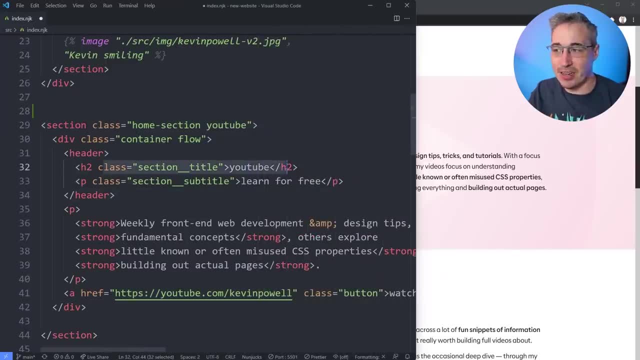 would work, but in this case, instead of using a title on my own page, what would actually make more sense is to come and reference the h2 that's here, and so to be able to do that, I would have to come and give this an ID. so ID is going to be, and I'll give this one the the ID of YouTube title, and so here on. 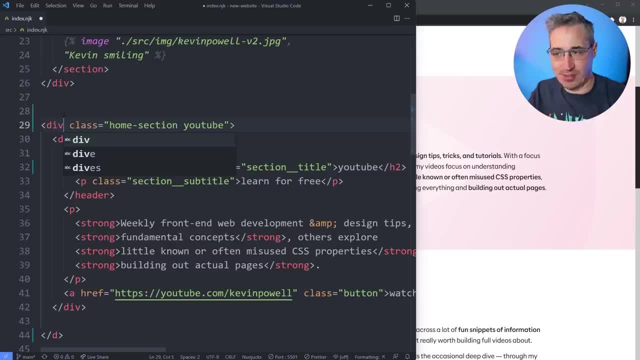 the section if I wanted to make this not you know, right now this is the same as having a div here. there's literally no difference between the two of them. but by coming and if I want this to, like semantically, be a section that's going to be a region on my site, I would then come and say area. 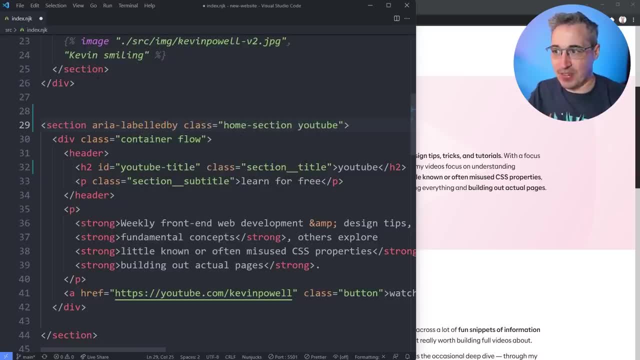 labeled by. and I've always found the labeled by a little weird. we're, you know so, used to having hyphenation. but anyway, area labeled by, and it's going to be equal to, and my YouTube title. and then I could come and I'd want to do the same thing. we can even go to my 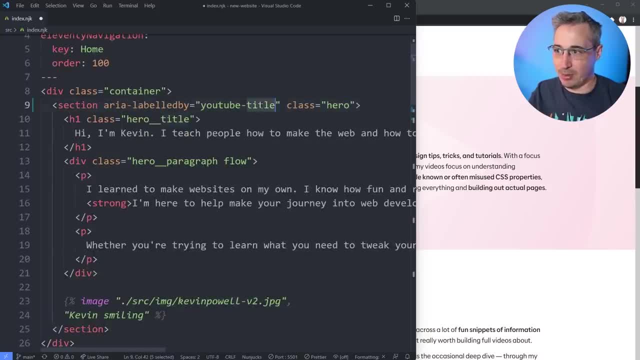 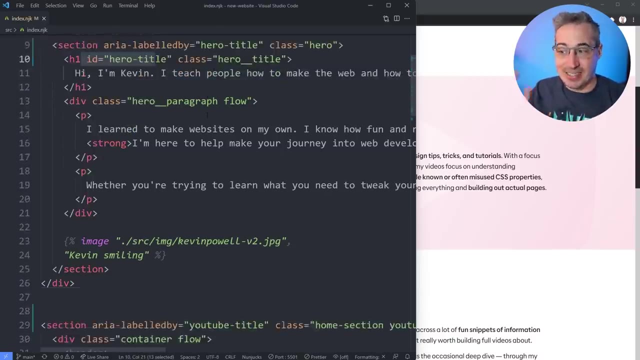 hero section at the top here. so this section will be labeled by my hero title and then we could actually just copy that and put an ID on here of hero title. and that, labeled by and having the ID on here, it links the two sections together. sections should, to begin with, always have a heading in them anyway, but if for some reason, 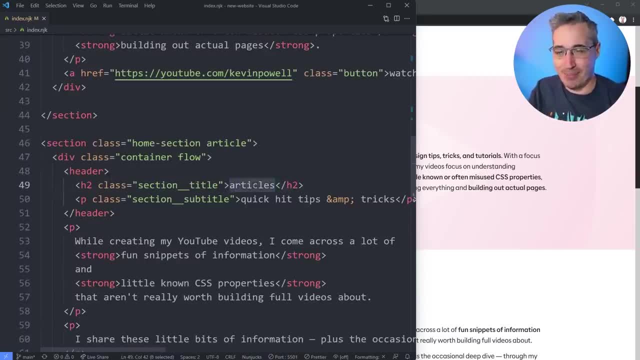 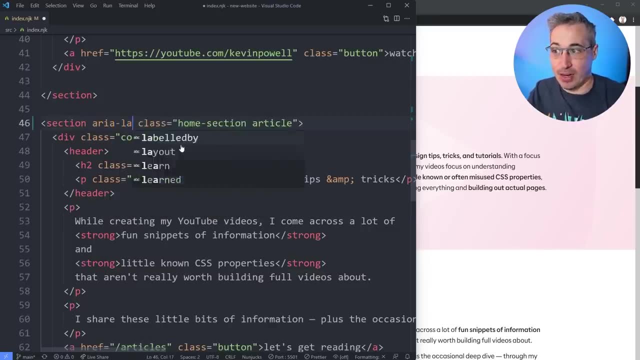 you think there'd be a better title or this doesn't quite describe in the way that you'd want to. um, you could come on this section here and give this a instead of an area labeled by. you could do the area label instead and say: and I could do articles here, um, in this case I think 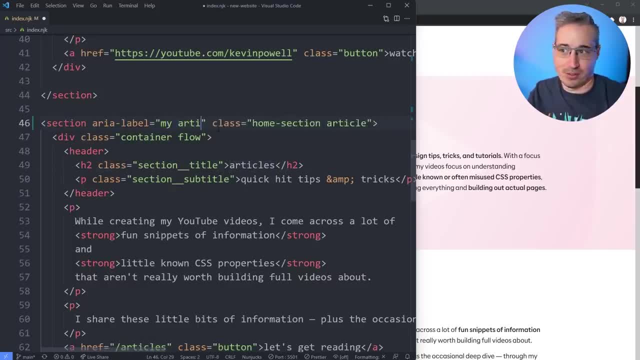 this title is fine, but like I don't know, I want a different one. my articles, let's say. and now this becomes the label for that entire section. now this also has the role of region on it, because I have this area label, or I could do it with a title, or I could do it with my area labeled by and just make. 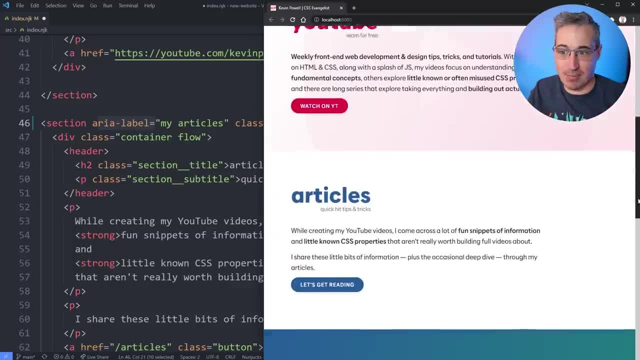 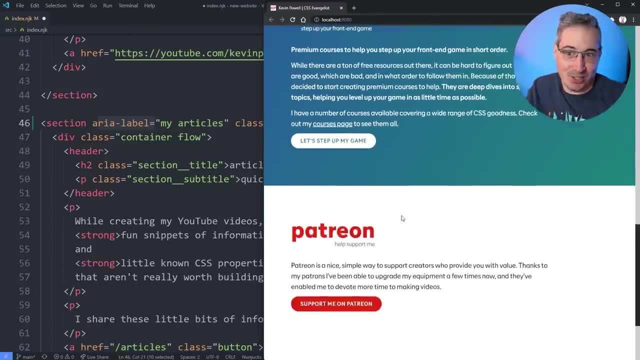 sure, if you have sections- and I think they actually do make sense on my site, how I've set them up on this page- because this is all part of my main here is about me, and then this like the different sections of this page- to me sort of do flow. so in this case I'm going to finish updating. 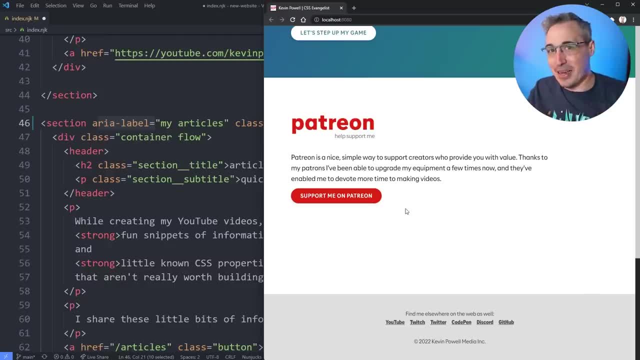 my site and I'm going to push this, and it just means you know, whenever we're writing semantic HTML, you do want to put a little bit of thought into it, and sometimes it's things like sections that you think work in a certain way, that actually work in a different way, and if you'd like more. 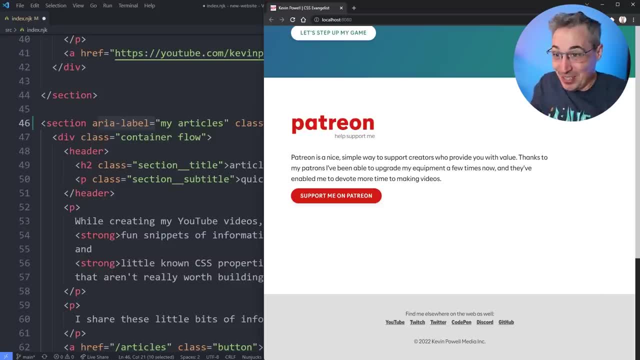 things that people get wrong when they're writing their HTML, uh, including some really simple things that you think we'd be getting right all the time. I have a video right here that you can check out, and with that, I want to say a very big thank you to my supporters of awesome over on Patreon: Jan. 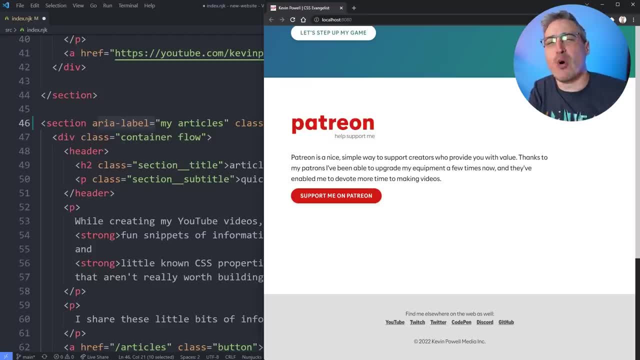 Johnny Stewart and Tim, as well as all my other patrons, for their monthly support and, of course, until next time, don't forget to make your corner, the internet, just a little bit more awesome. you.